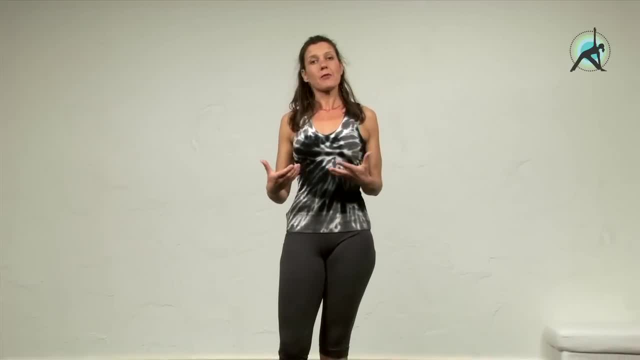 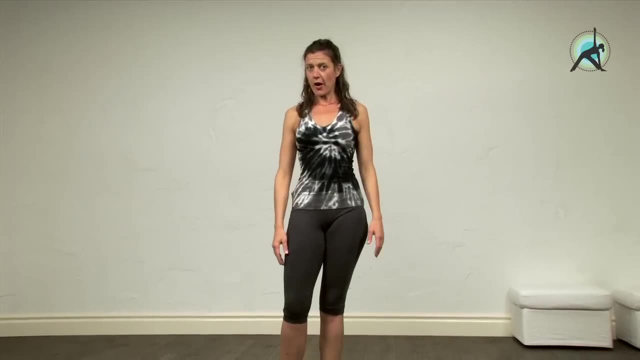 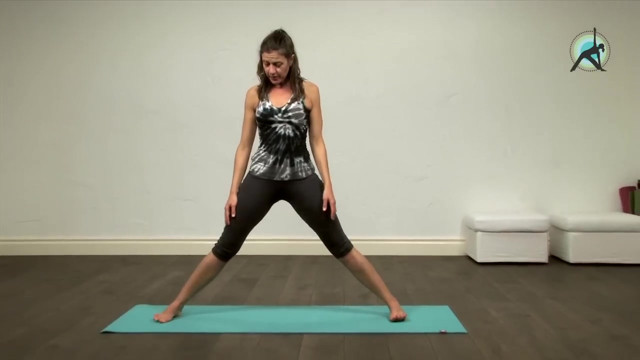 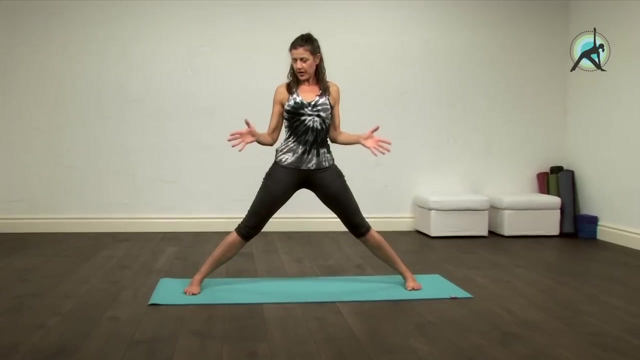 And you can incorporate these into your daily practice, into a more dynamic, into a dynamic flow. There are many elements that can be incorporated into different way of practicing, So we'll start with a nice wide stance. I like to start with, yeah, quite wide feet, Different levels. if you're new to this, you may want to have your feet slightly closer. 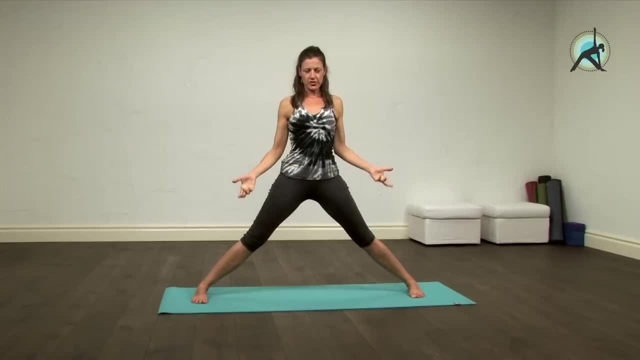 But it's important to cultivate already the foundations Which are extremely important, especially in standing poses to protect knees and joints in the lower body. So the feet are really strongly gripping into the floor. The outer foot is strongly pressing the inner and outer heel and the ball of the big toe. 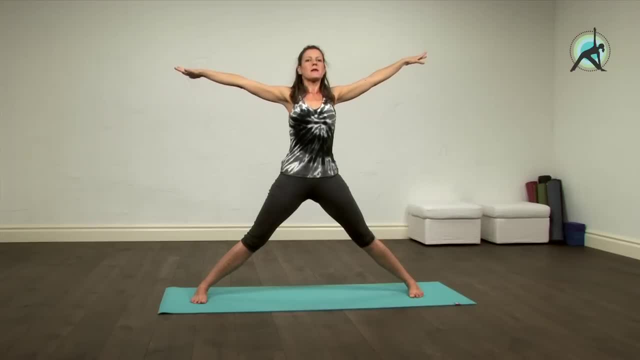 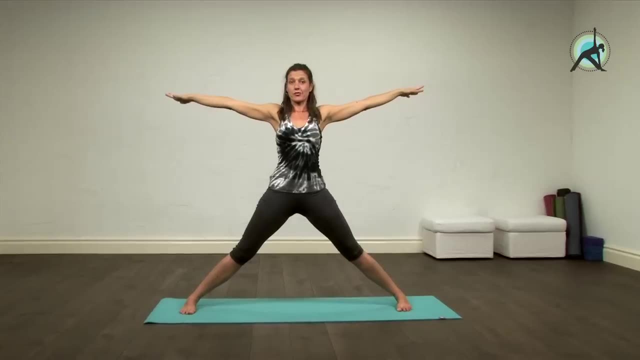 Now we'll start with the arms already. So the shoulders: there is an element of softness in the shoulders, So see that you're ready, you're not clenching, And if you're finding that your arms are getting tired throughout the practice. 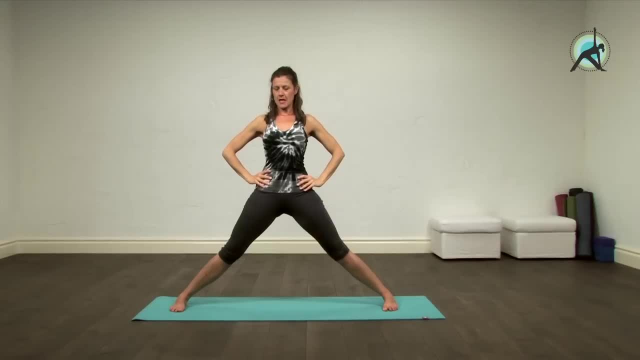 please have them onto the head And the hips. that's perfectly fine at any stage. So, with the arms out, we're going to start with the right foot turning out, so the heel can press on the floor and we're moving to Virabhadrasana. 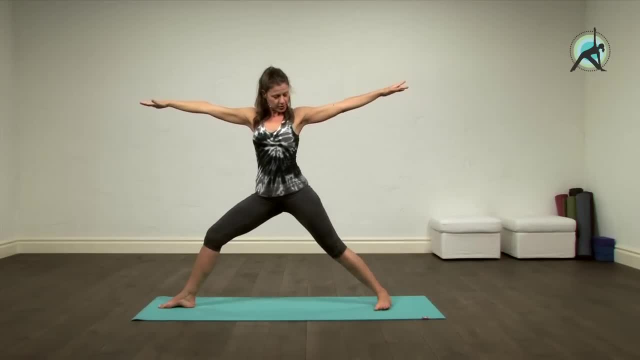 So we can bend the right knee. The back toes can actually turn slightly in as you do this And, as you can see, the right thigh will be parallel with the floor. Hopefully it will be parallel with the floor. with practice, The right knee will be in line with the ankle. 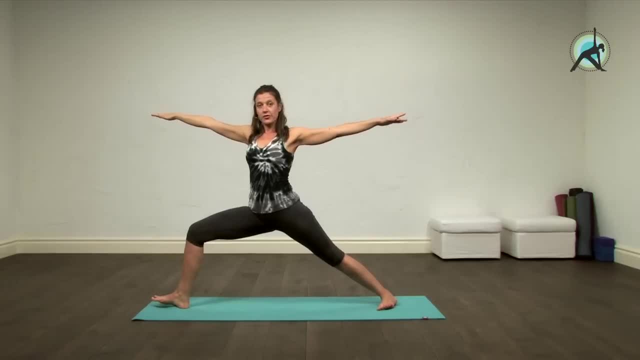 And you can also add an element of softness. You can also add an element of strength by pressing onto the right heel strongly. So remember, you're anchoring with the back foot, So the back foot is what keeps your alignment. So, Virabhadrasana 2, you can do the pose with the version where the palms face up. 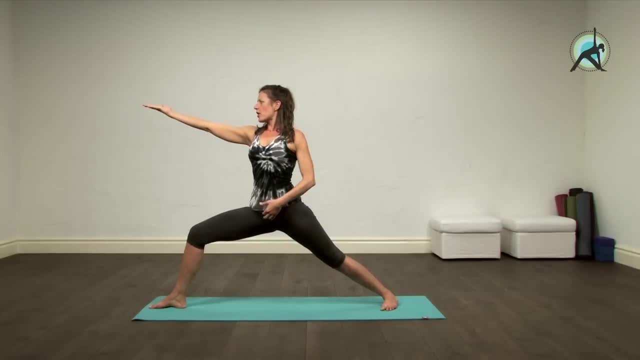 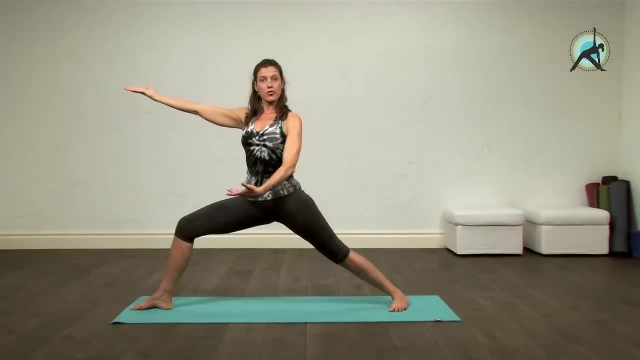 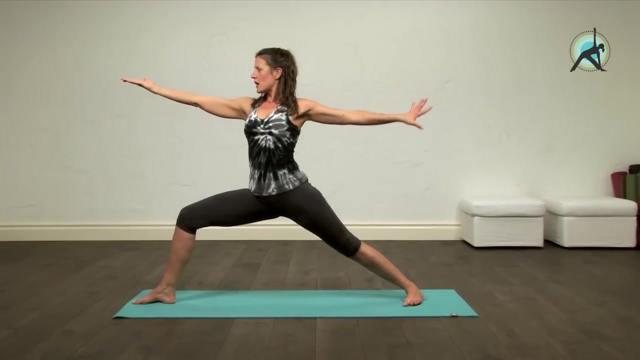 The tailbone drops down And you want to add the element of the pubic bone moving in towards the sacrum, This area gets kind of shorter, So there is no dropping of the organs forward From this position. keeping all these elements, if you can, you want to start to drop your left arm down, the left hand down to the left leg. 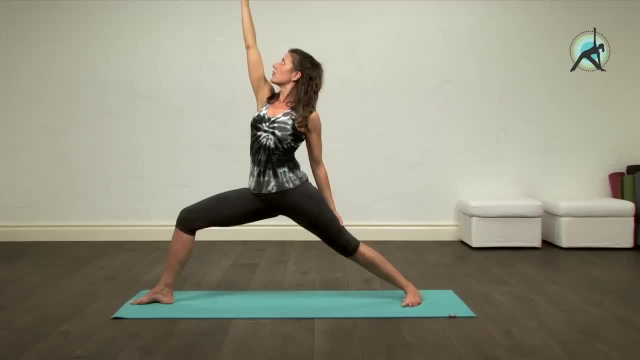 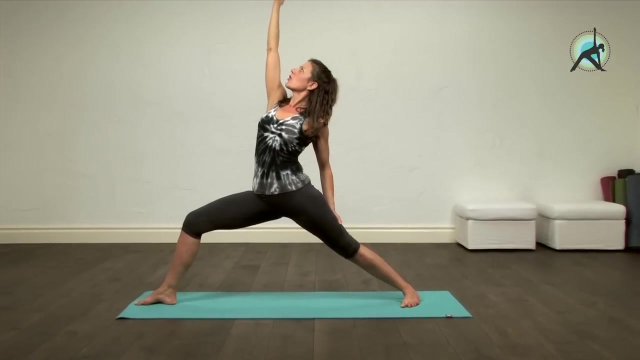 And gently start to raise up your right arm. You can follow the right hand with your gaze or you can gently gaze straight ahead, Sending the tailbone down and keeping the lumbar spine open. You want to keep the chest lifting, Creating a sense of opening into the collarbones as you gently slide your hand down into your left leg. 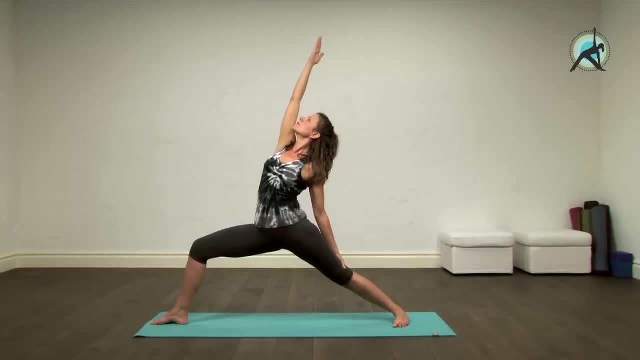 Opening the heart, softening the gaze. You can take a couple of breaths here. Remember to connect with your feet and to your front knee. The front knee stays bent. Move your heart up. Try not to sink into the lumbar. 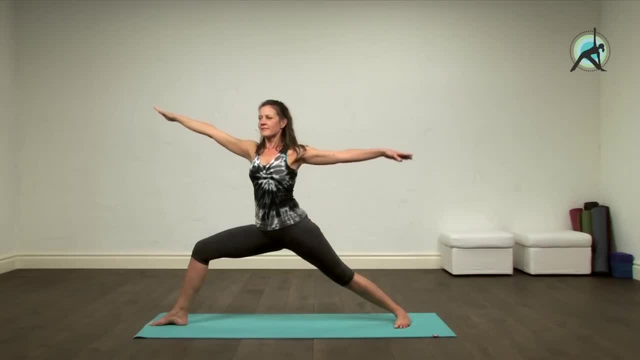 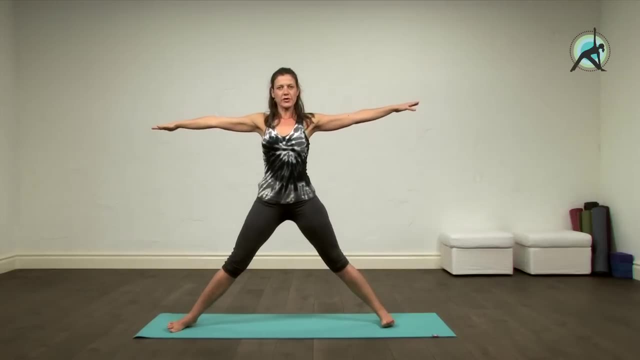 And, as you breathe in, come to the center. We're going to straighten up the front knee and bring the feet parallel in your own time, in your own way. If your knees, if your ankles are a bit tired, okay, you can maybe bend the knees. 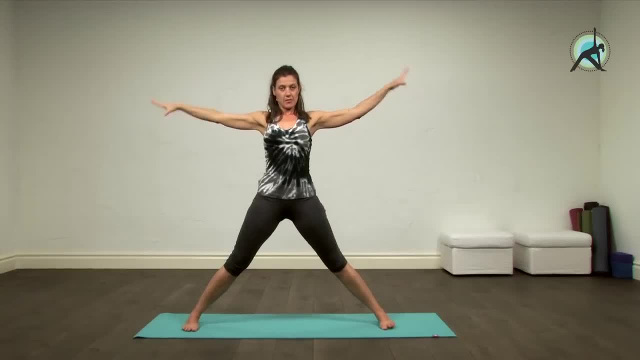 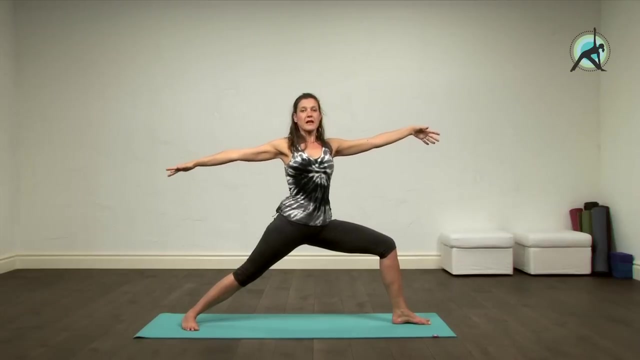 Changing sides. Remember to have your hands on your hips if you need to, Right toes in and left toes out. Bend your left knee Into Virabhadrasana. Yeah, fine, I like to have. I like to slide my foot slightly more forward to have the correct alignment. 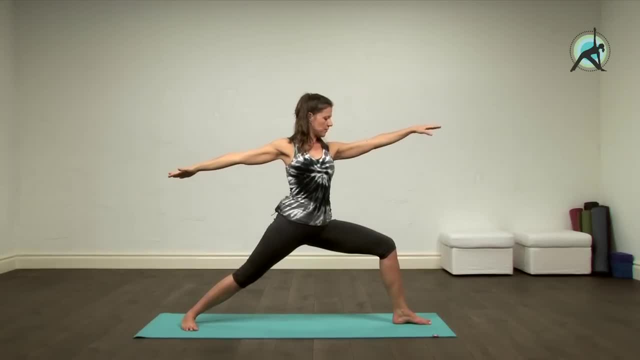 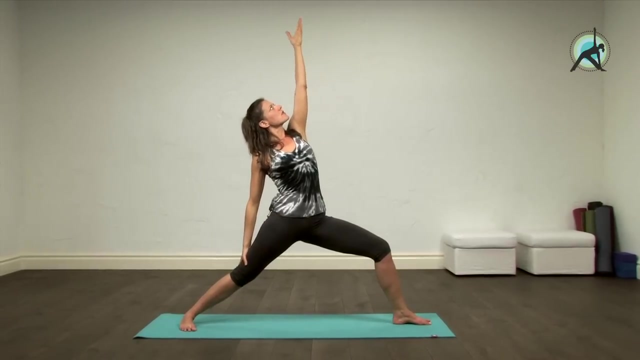 So you can use your gaze, You can use the physical body, the physical gaze okay, to really align your body And as you connect with the back foot, you can start to lengthen and to send the tailbone down. At the same time, the pubic bone moves towards the navel as you stretch your left arm up. 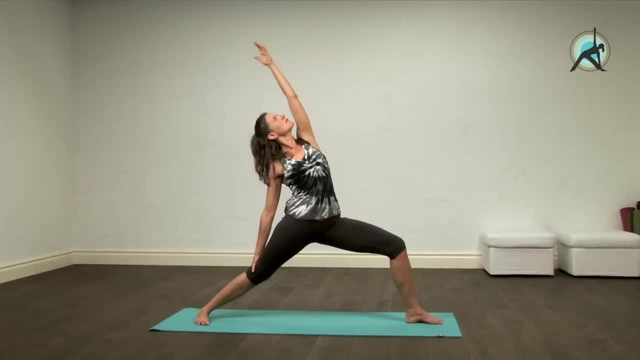 The back leg can be strong. Remember the element of lifting from the heart, keeping the collarbones nice and open, And as you breathe out, come to the center, Connect with your both feet And then straighten up your left knee. 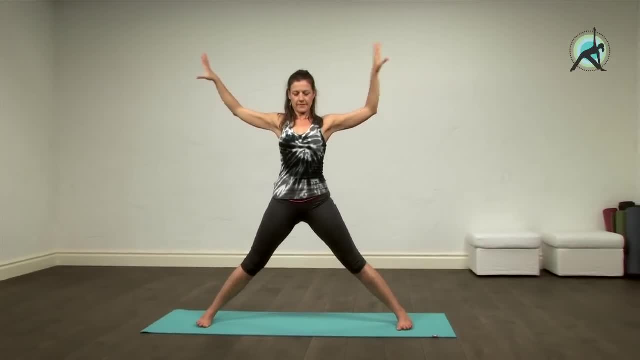 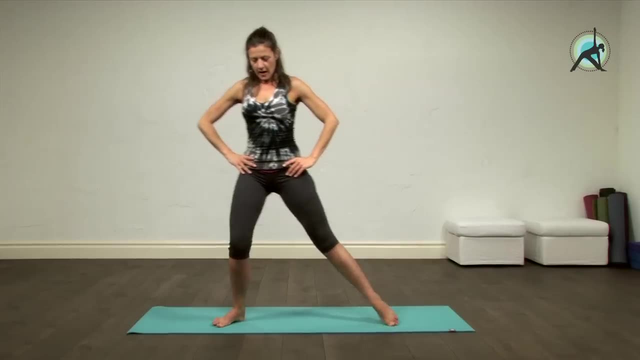 Your toes pointed, Your toes point forward And hands on the hips. again, You can either walk your feet or jump them together if you're used to jumping, And there is a beautiful element of chest opening, of course, into Virabhadrasana.